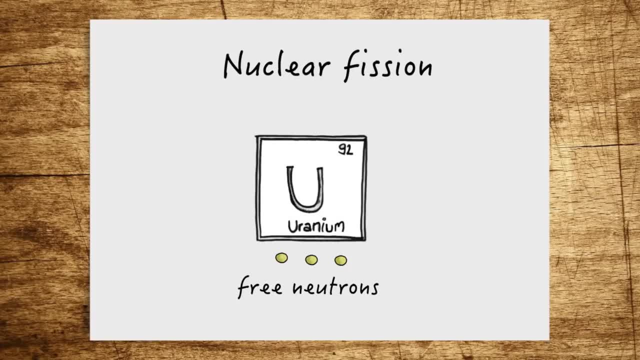 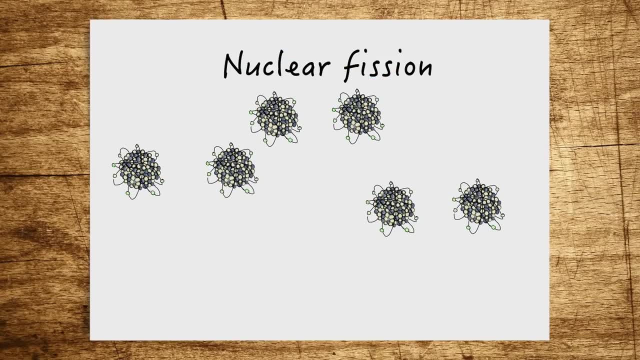 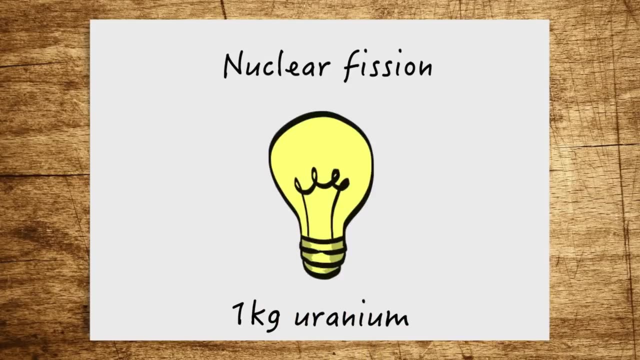 When uranium atoms are split in a nuclear power plant, this usually involves the release of three neutrons. These can then affect the next fission processes in a chain reaction And finally energy is released, And very much of it at that. One kilogram of naturally occurring uranium has the energy of 12,000 liters of mineral oil. 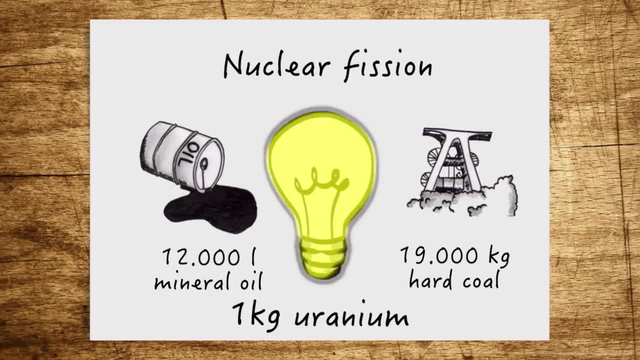 Or of almost 90% of it, 19,000 kilos of hard coal. But where does this energy come from And why is it so much more than in the case of other energy carriers such as oil and coal? Let us recall: 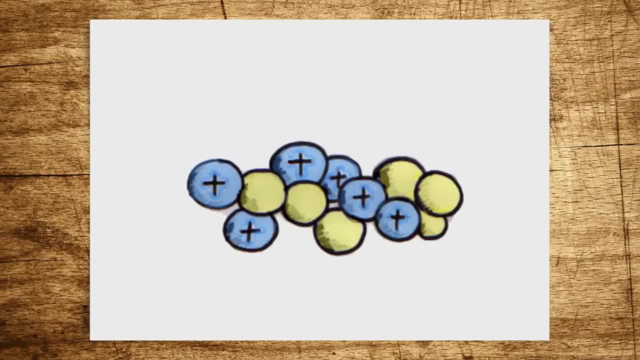 Besides the neutrons, the atomic nucleus only consists of the positively charged protons. Now, equal charges repel each other, Similar to the equal poles of two magnets. The fact that the protons in the atomic nucleus remain together nevertheless is due to the so-called strong interaction. 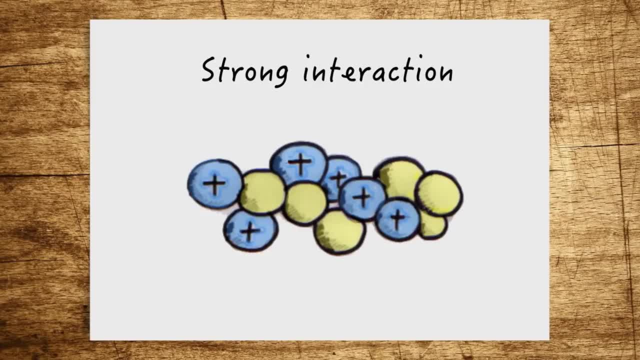 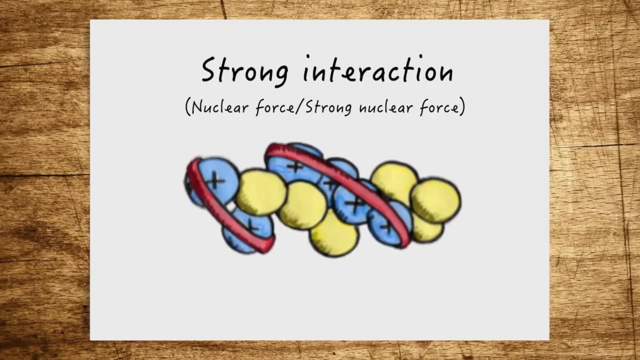 This is one of the four factors. There are fundamental forces in the universe, and by far the strongest. By the way, this force used to be called nuclear force or strong nuclear force. It acts like a strong rubber band that holds together the atomic nucleus with its protons. 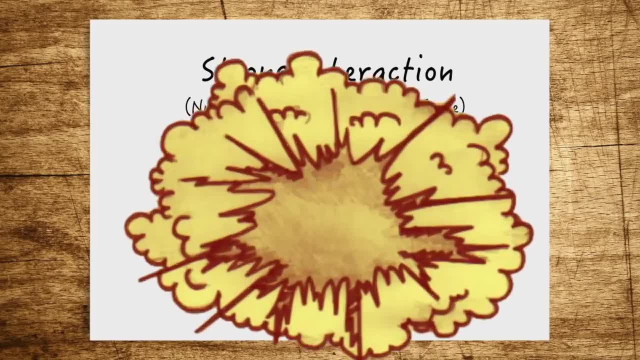 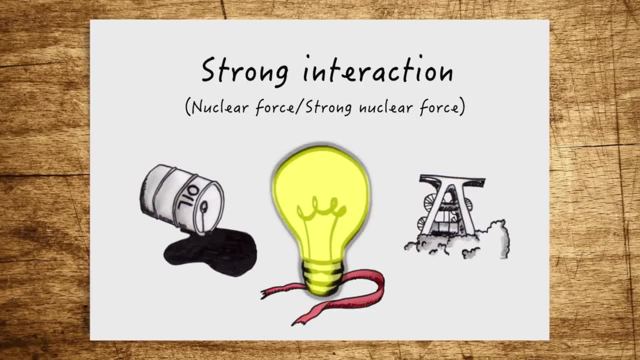 which we know do not really want to hang around so closely together. When the impacting neutron forces the nucleus apart, it is exactly the energy that has been stored in the rubber band that is released. This energy is not released upon the burning of coal or oil. 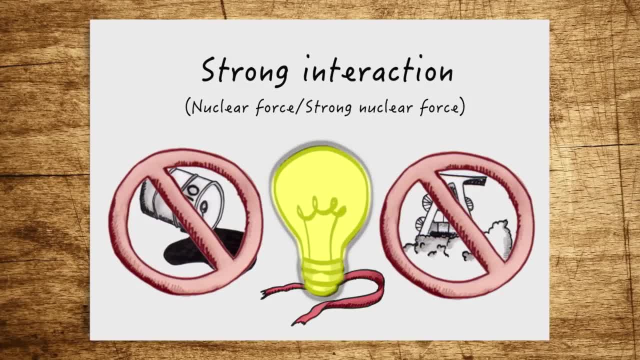 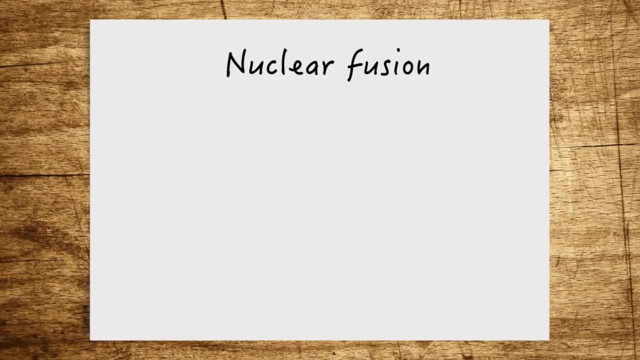 In this case, there are chemical reactions developing in which the atomic nuclei are not touched and where only electrons are exchanged. Nuclear fusion presents a similar picture, Or rather a mirror image. It only works with small atoms, like hydrogen, for example. 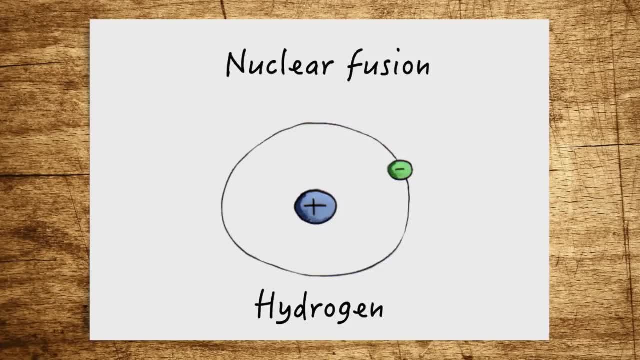 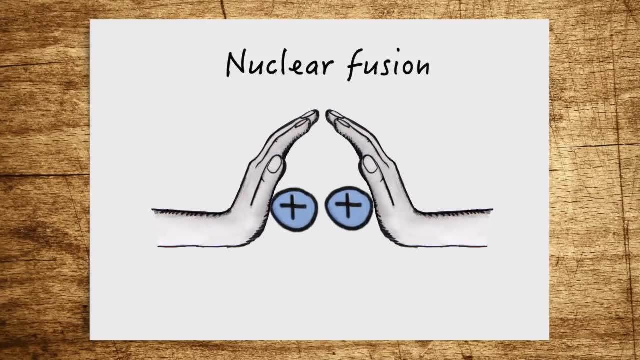 The atomic nucleus of the latter consists of only one proton. If one now tries to force two of these protons together, these two would have to repel each other due to their equal charge, as in the case of magnets. When talking about atomic nuclei, this is referred to as the so-called Coulomb force. 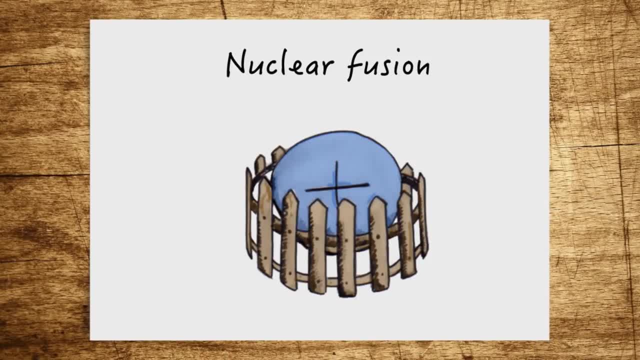 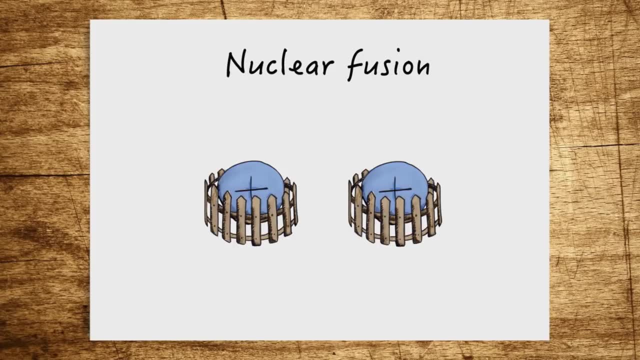 This force acts as if each of our protons had a fence around it, trying to keep off other protons. Like fission needing a force that overcomes the rubber band of strong interaction, fusion also needs one that forces the protons so closely together that the fences are pulled down.